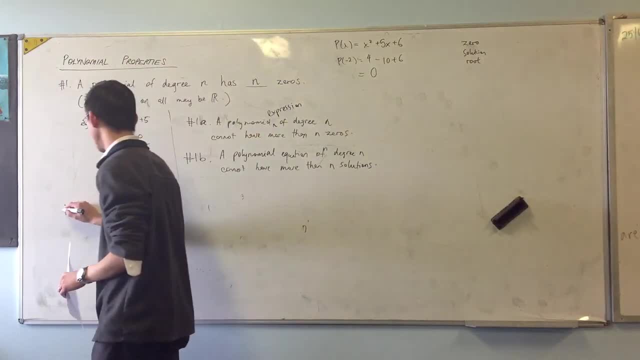 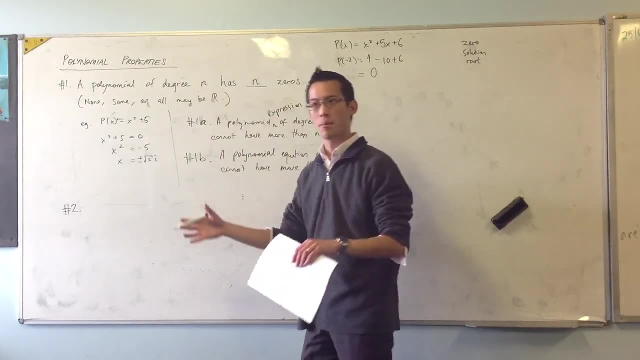 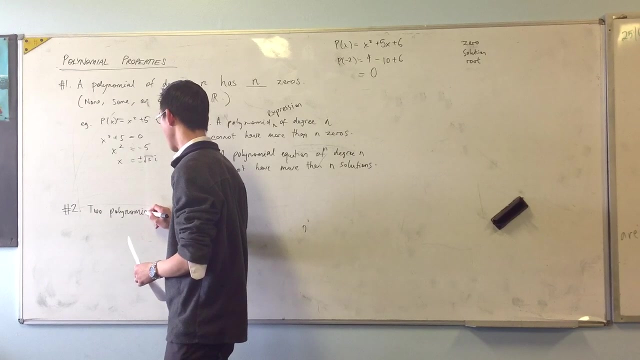 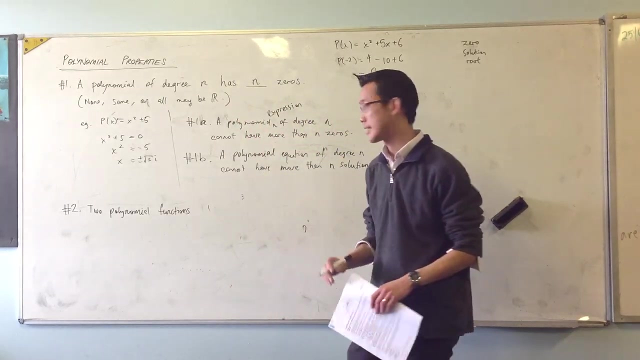 Okay. now number two: What happens when we've got multiple polynomials, and how can we? is there an application of this to having more than one polynomial, mainly two. So if I say two polynomial functions, okay, and if I'm interested in how many points they intersect at, okay. so this is going to be a direct flow, one from one b, okay. 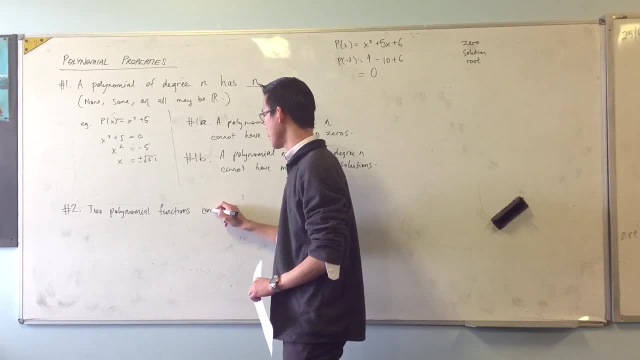 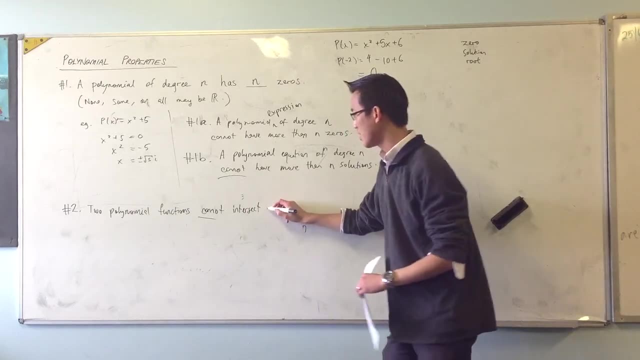 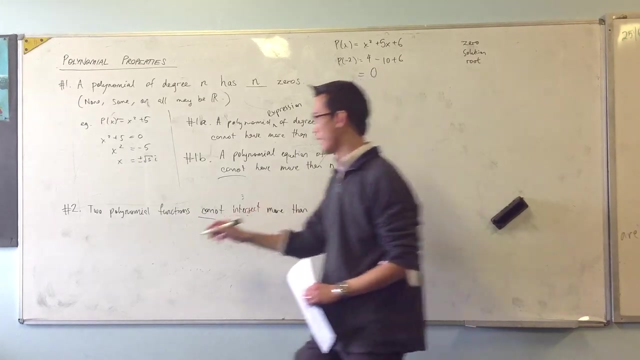 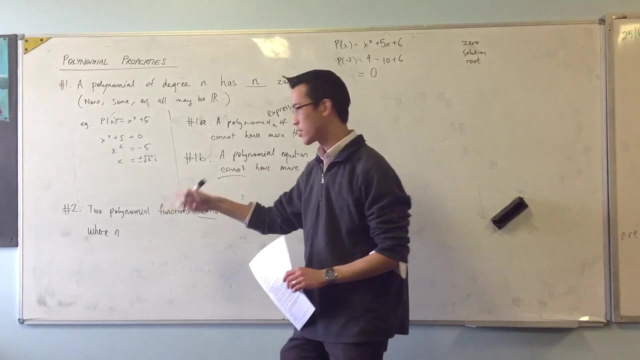 Two polynomial functions cannot intersect. so you've got this same cannot language, right, and they're parallel. cannot intersect more than n times. where now, what's the significance of n? You can actually have the polynomials having different degrees if you like, but n is going to be where n is the degree of. 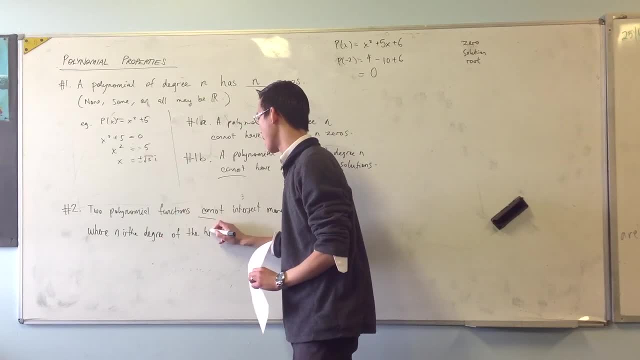 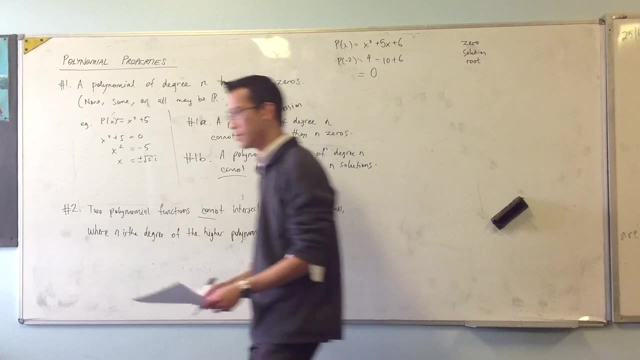 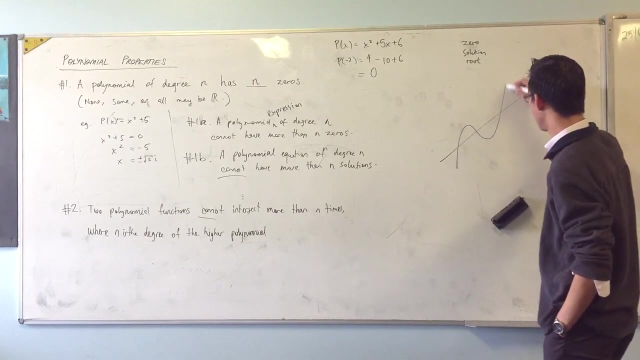 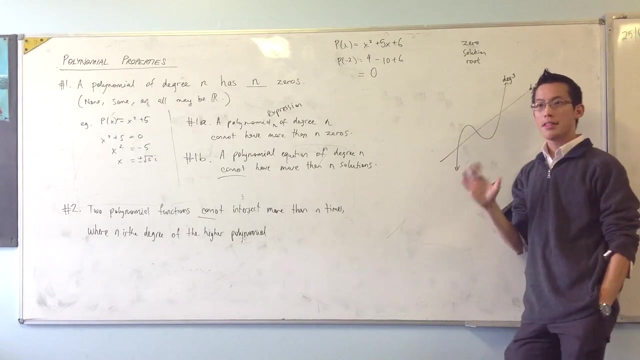 of the higher polynomial. okay. so by higher I mean it has a bigger degree, okay. so if I gave you a simple example, okay, like say, a straight line: okay and a cubic, degree three and degree one: okay, there's going to be at most three points of intersection which you can actually see here, right? 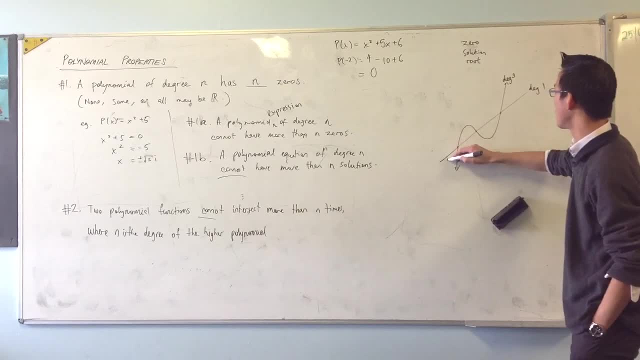 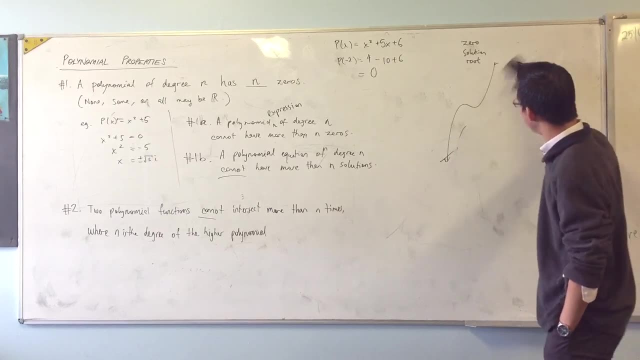 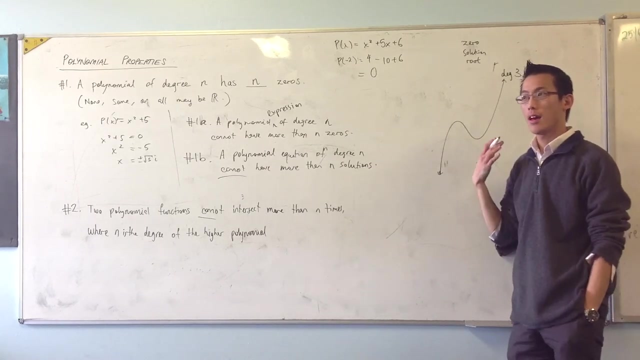 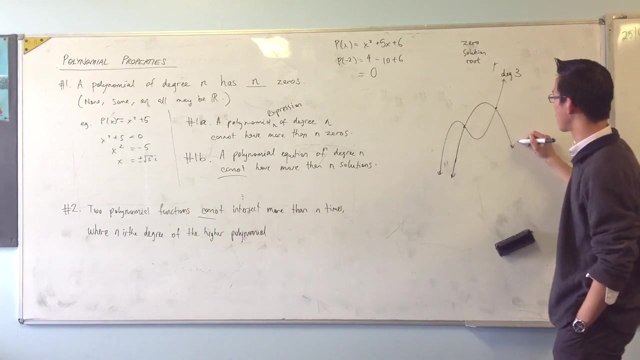 there might be less, just like I rubbed it off, if I moved it up again. okay, there may be less than three points, but it can't be more. okay, in the same way, if I took a cubic- degree three, right- and put it together with a quadratic- okay, so degree two- okay, in this case, the one that I've drawn. again, I've got two points of intersection. I could draw one which was maybe flatter. 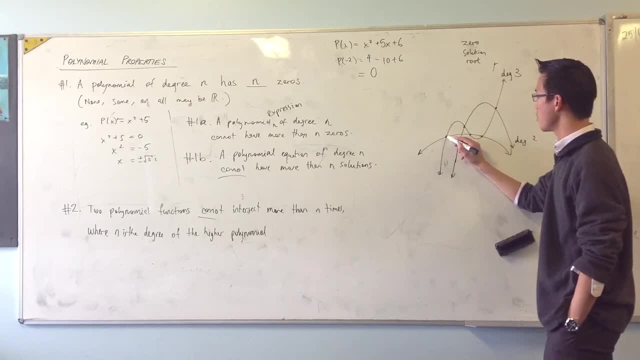 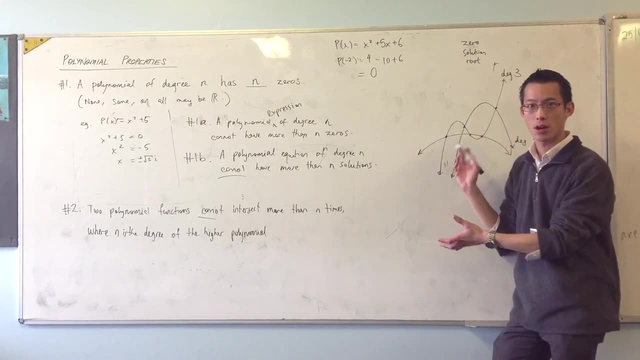 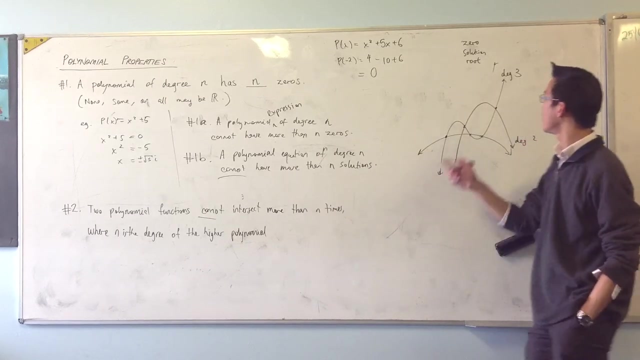 and had three points of intersection, but there's no quadratic I could draw that would intersect with the cubic four times. okay, because it won't match up with the degree that I've got now. can anyone see why, and can anyone particularly connect it back to 1b? why is it that if this degree is three, I can never get more than three points of intersection with any other graph? 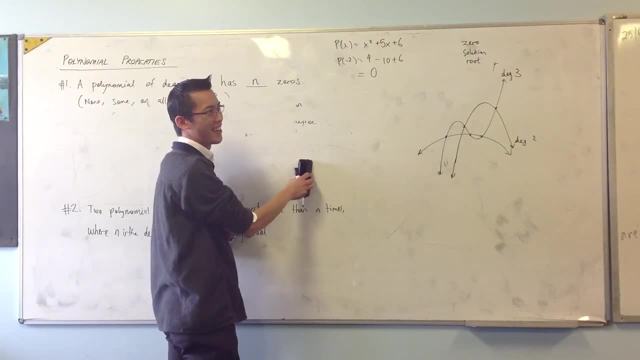 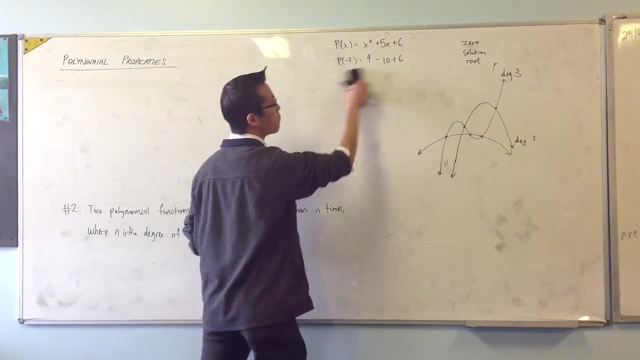 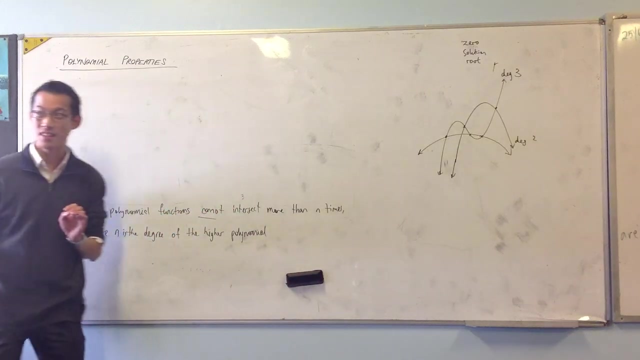 Polynomials, polynomials by definition. polynomials just has the, just has the one variable. so yeah, any other ideas, apart from seeming contradictions of this? okay, let me try to explain with an example. okay, so let's have two top polynomials. okay, let's go with the x cubed. 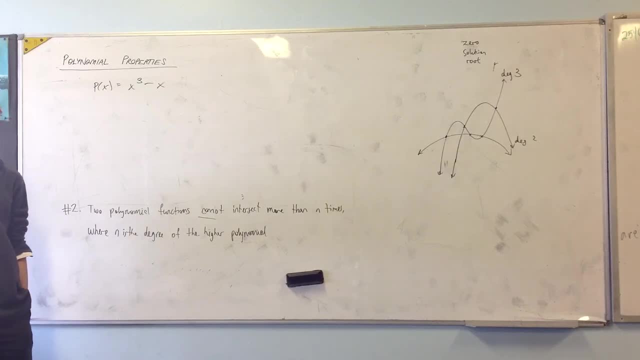 minus x one that I had before. okay, and let's see how many times it intersects with a line like say: oh, I don't know, two x plus one. okay, now to find points of intersection between two graphs, what do we do? 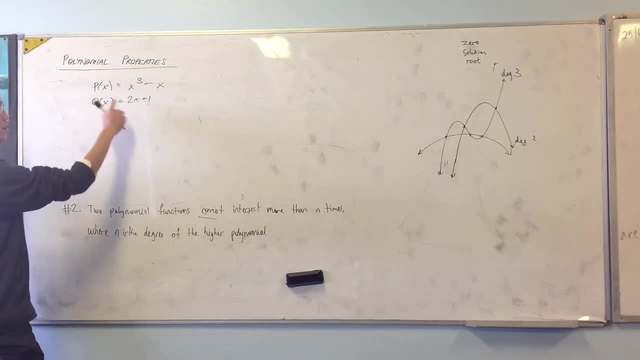 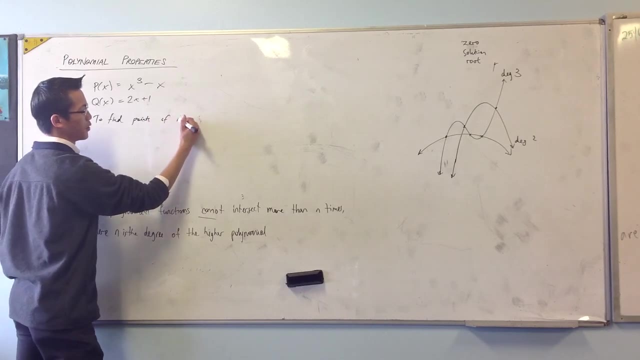 Yeah, that's right. you let one equal the other. okay, so I'll say p of x equals q of x to find points of intersection. yes, thank you, I'm here all week. I'm going to let p. 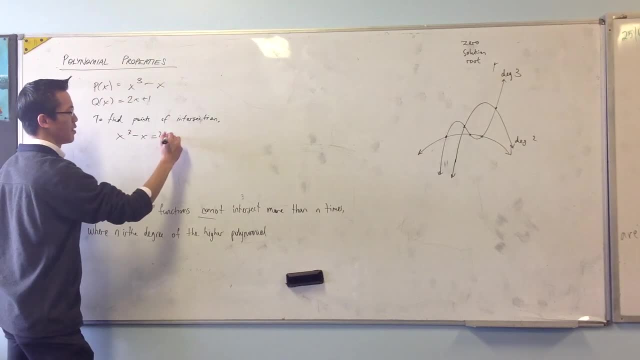 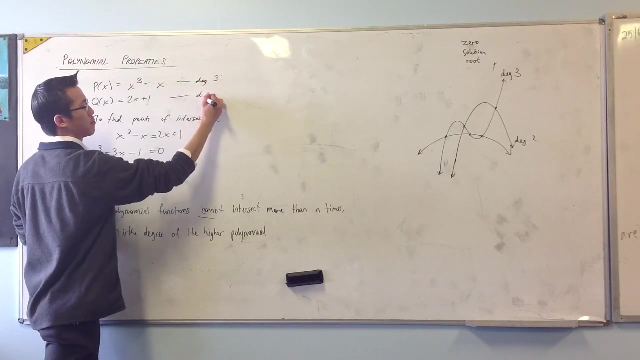 equal q. okay, so x cubed minus x equals two x plus one. all right, now, when I go ahead and solve this, I mean usually we take everything over onto one side, so I'll get x cubed minus three, x minus one, and then I go ahead and solve that, right? ah, can you see what's just happened? right in solving a polynomial with degree three with a polynomial degree one. okay, to solve them. the way that you do it is you create a new polynomial. 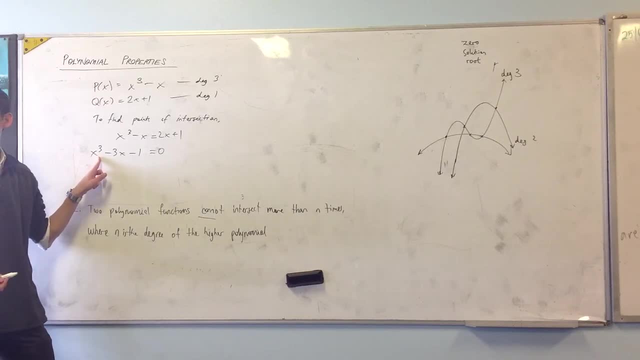 okay with degree three, namely, you got it from here, right. and of course, if this is degree three, then from property one b. I think that's one, right? it can only have a maximum of three solutions. there's only ever going to be three solutions to this and, of course, solutions for this thing, right? what that really means is points of intersection. okay, so can you see how one flows onto two, right, that's the maximum number of points of intersection you're going to get. you might have less, but you can't have more.